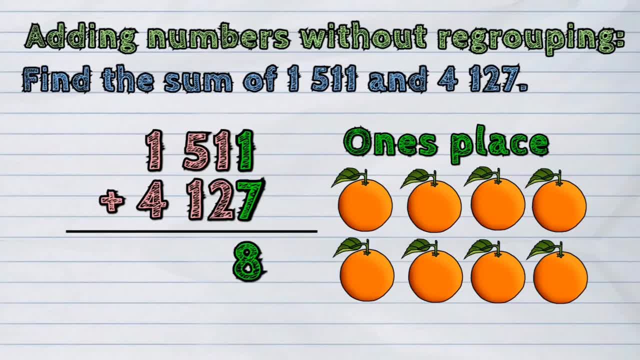 And next, we will add the digits in the tens place. 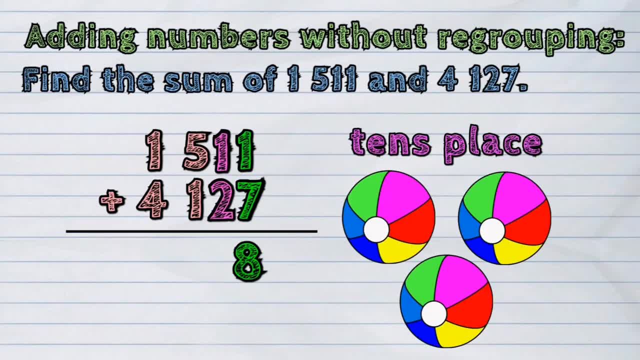 Adding 1 and 2 gives the sum of 3. 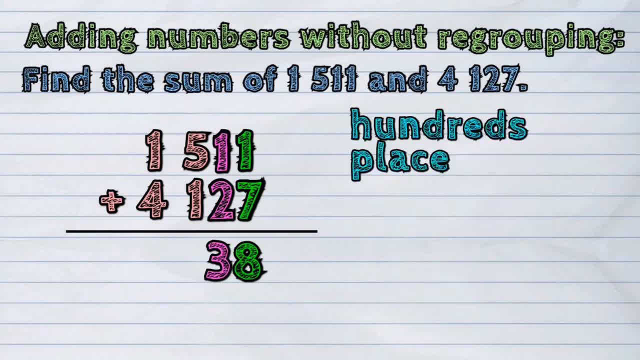 Now, let's proceed to the digits in the hundreds place. Adding 5 and 1 gives the sum of 3. 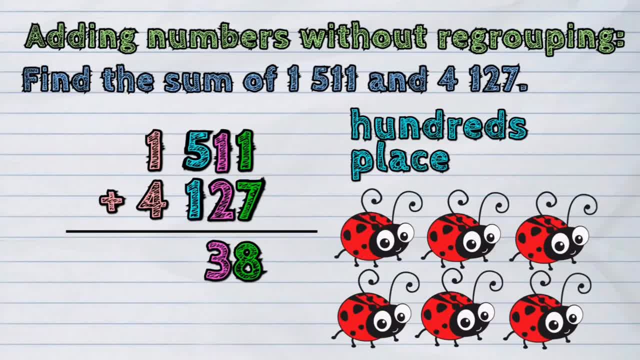 Adding 5 and 1 gives the sum of 3. Adding 5 and 1 gives the sum of 3. Adding 6 and 1 gives the sum of... 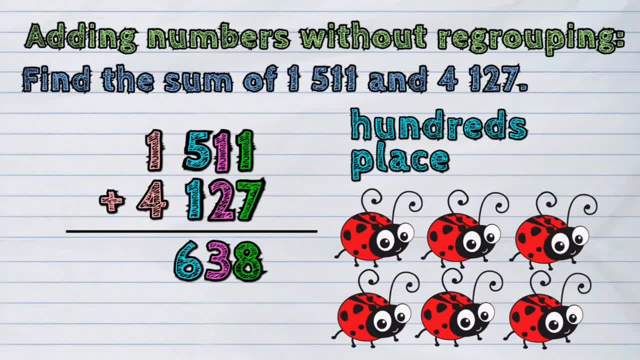 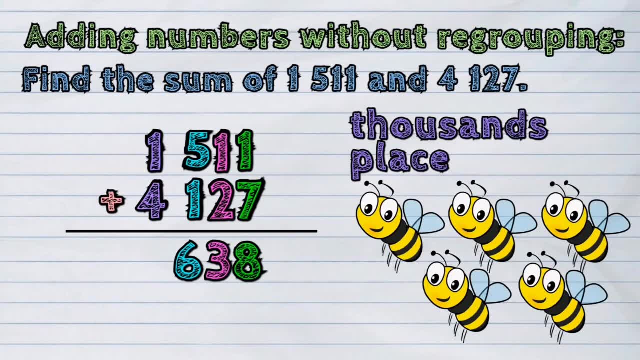 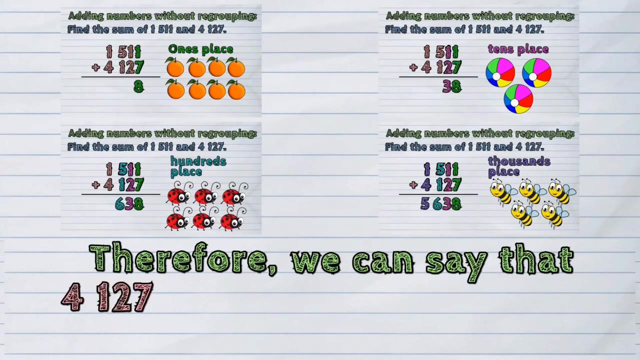 6. Adding 5 and 1 gives the sum of 3. Lastly, the digits in the thousands place. 1 and 4, when added together, gives the sum of 5. Therefore, we can say that... 4127, when added, is... When added to 1,511 is 5,638. 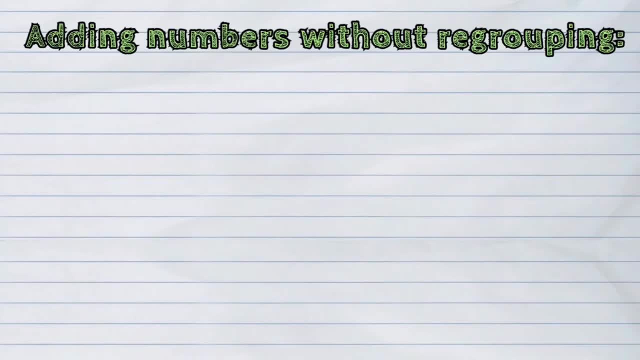 Let us take another example. Add 58,413 and 21,456. 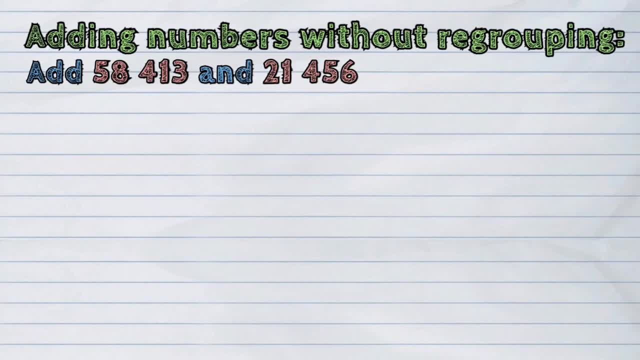 Again, we will write the numbers in columns. So, 58,413 plus 21,456. 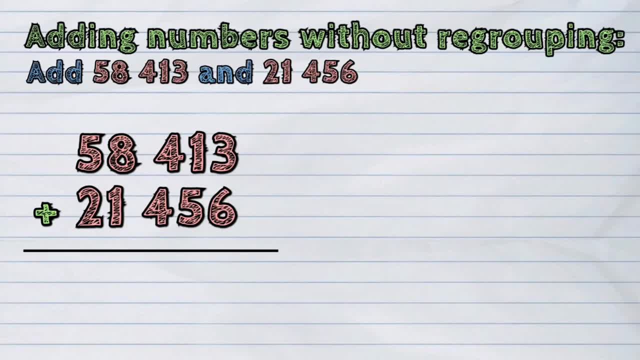 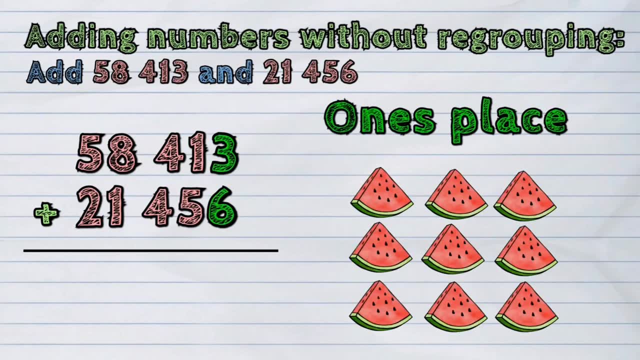 We will now start adding from 1's place. If we add 3 and 6, the sum is... 9. 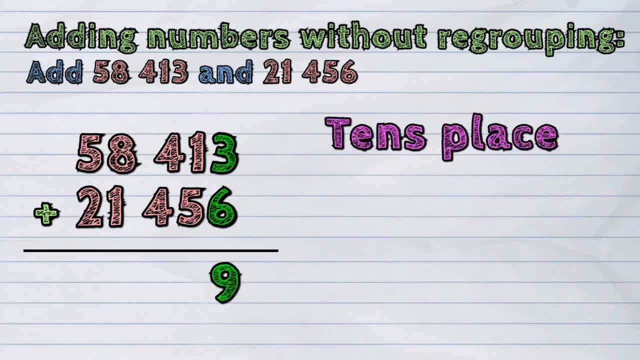 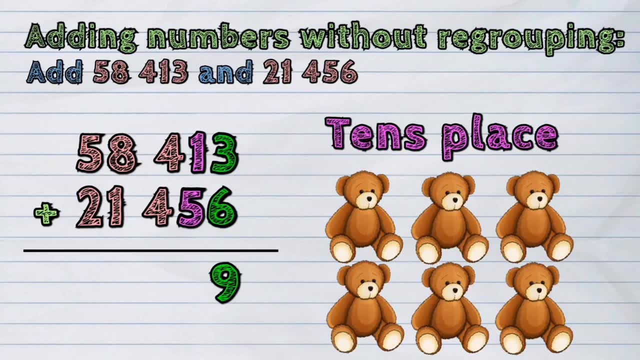 Now, we will add from the 10's place. Adding 1 and 5 will give the sum of... 6. 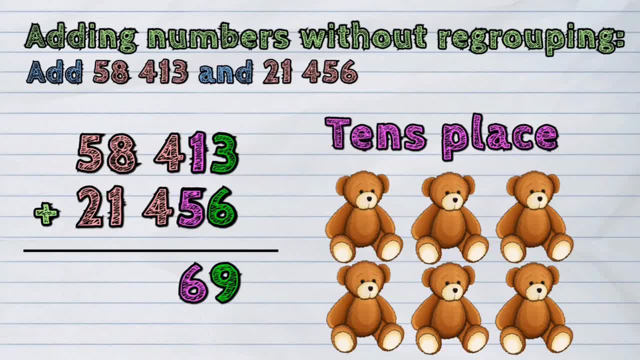 Next, let's add from the 100's place. 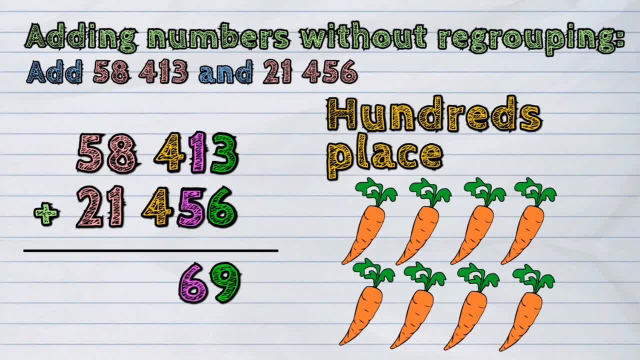 Adding 4 and 4 will give the sum of... 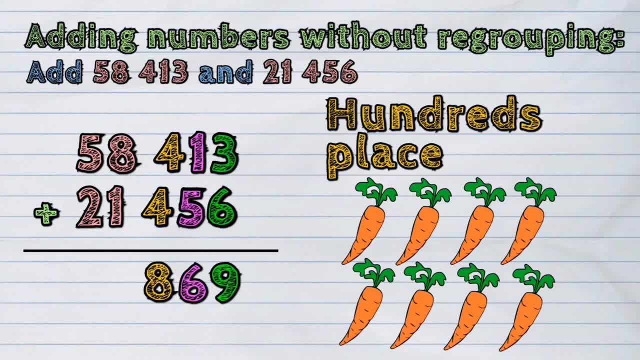 Next, from the 1000's place. 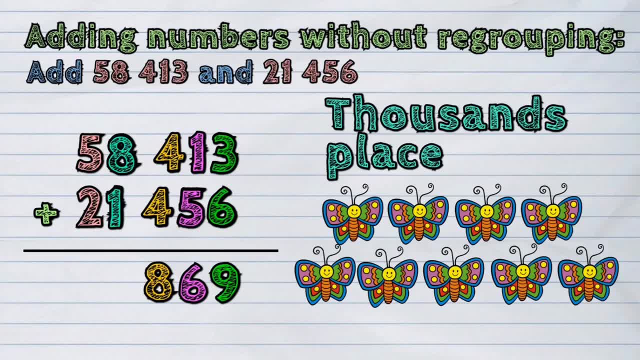 Adding 8 and 1 will give the sum of... 9.